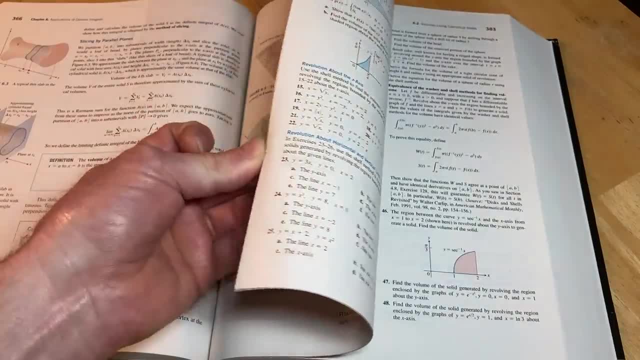 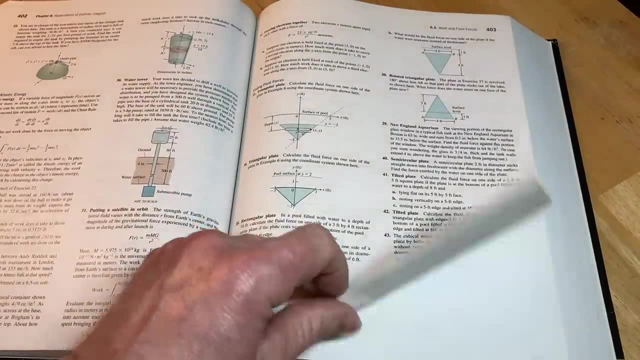 But this is a book that was recommended to me a long time ago. It's been a while- It's been a few years now- From subscribers here on the channel, In particular people from India. they mentioned that this was a book that they used, and so I went online and 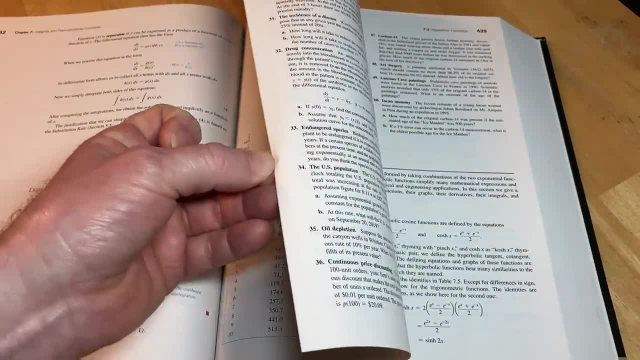 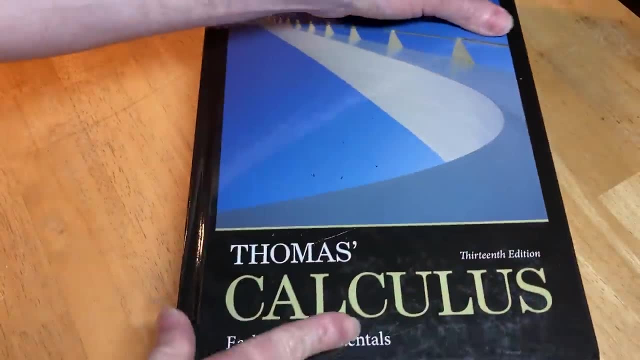 I did some research and I found it and I ended up getting various copies of this book. I actually have like three different versions. So this book is awesome and it is the one by Thomas. It's called actually Thomas calculus. 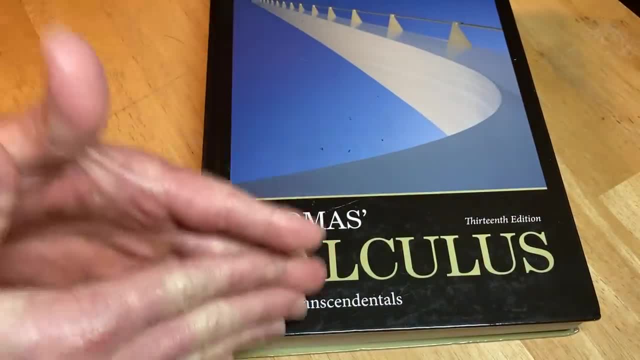 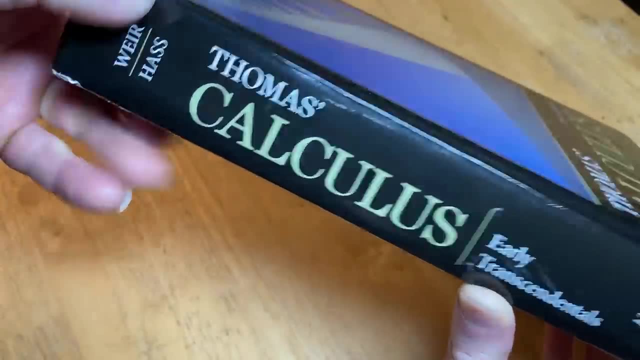 name is in the title right, So it's Thomas Calculus. It's the 13th edition and it's written by Weir and Haas, so basically revised by these people. Let me show you what I mean by that So. 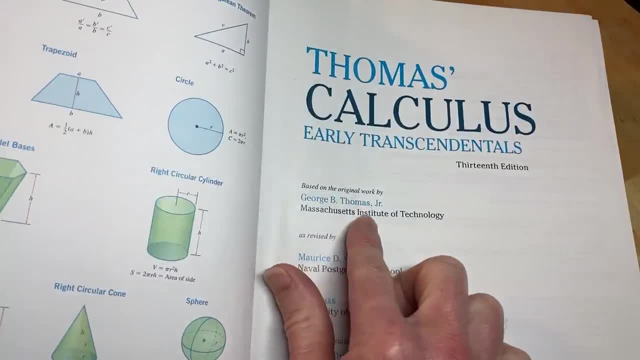 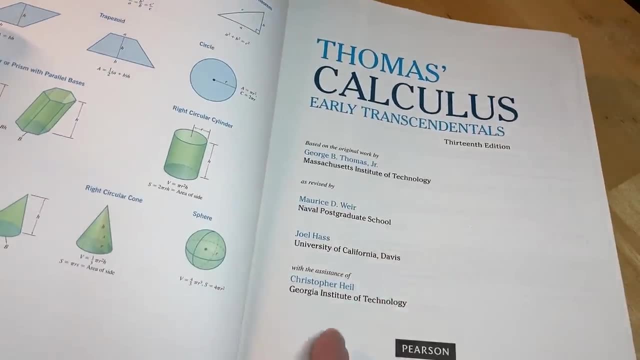 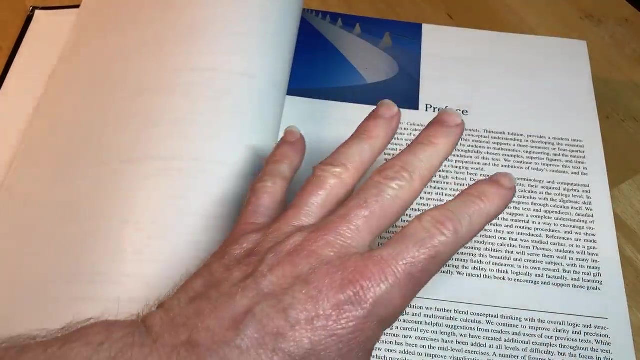 it's based on the work by George B Thomas, MIT, Massachusetts Institute of Technology, as revised by- and these people here revised it with the assistance of Christopher Heal, So it's a book that's withstood the test of time. There are major differences in newer versions of 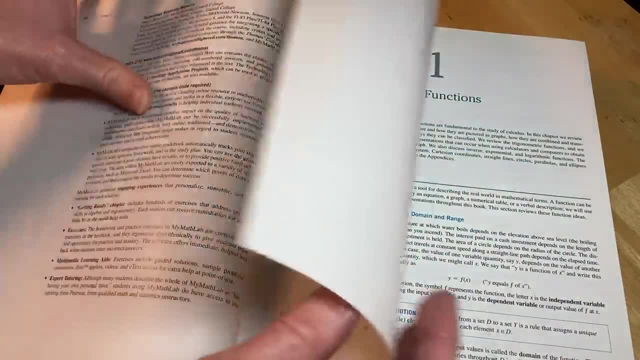 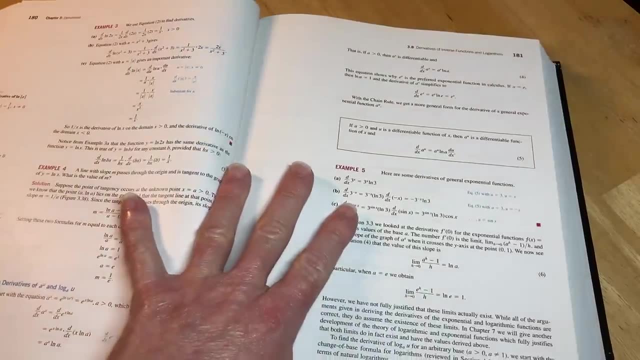 this book compared to older versions. In particular, a lot of the used versions, a lot of the older copies have answers to all of the exercises, whereas this one has answers to only the odd numbered exercises. So this book has everything. okay, It has everything you need for Calculus 1,. 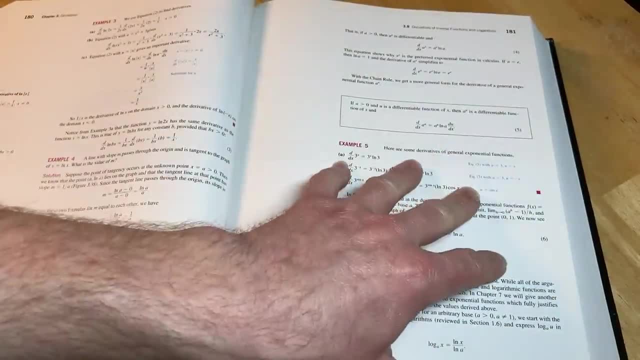 Calculus 2, and Calculus 3 in a college setting in the US. It basically has everything you need for Calculus 1,, Calculus 2, and Calculus 3 in a college setting in the US. It basically has everything that all of the other big, thick Calculus books have. It has 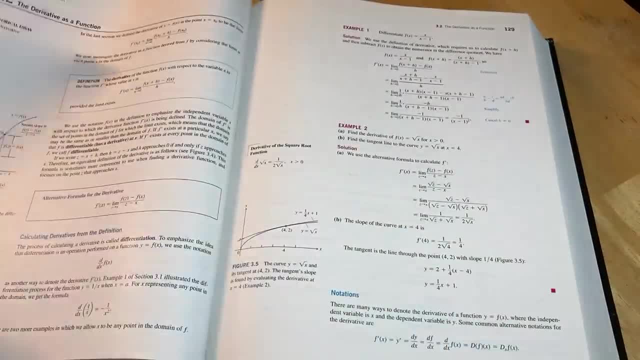 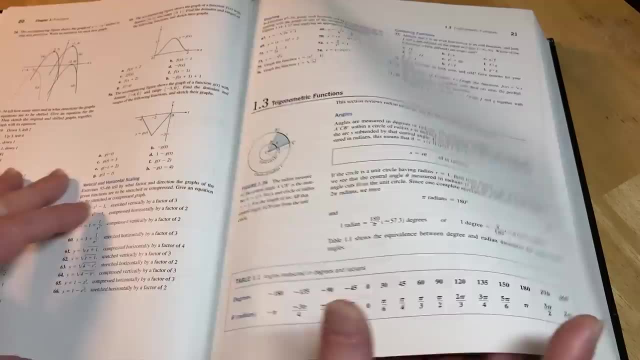 everything the Stewart book has, everything the Larson book has, etc. What makes it special, I guess, is that it's based on the work by George B Thomas. It's an older book, which was published a long time ago, and it somehow withstood the test of time, which is 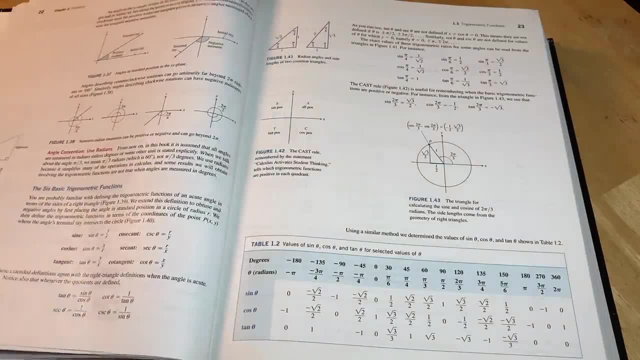 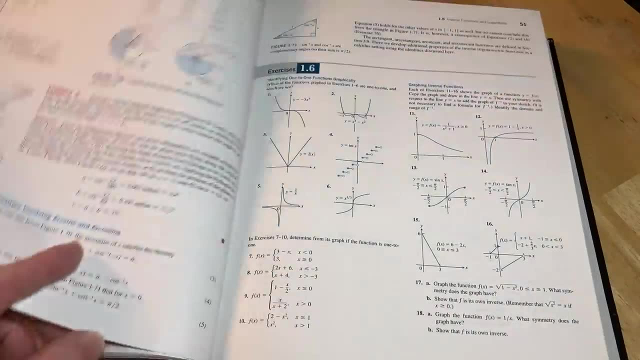 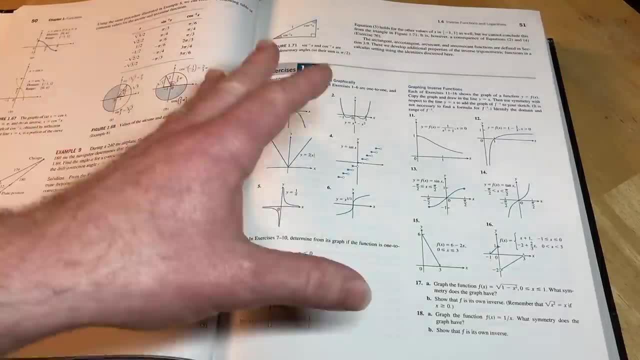 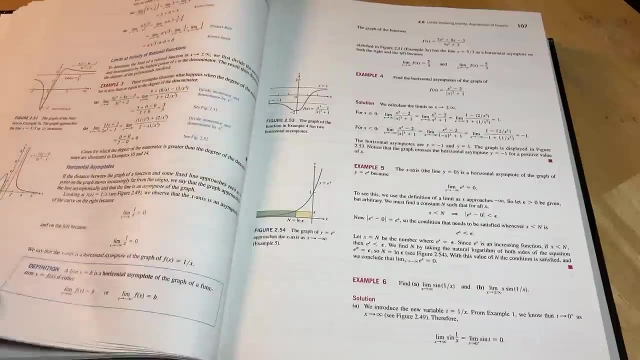 are that sometimes certain problems or topics were left out, and this one has additions to it that weren't in the old books. There are distinct differences and honestly I think both books were good. I'm not going to say that the new one is worse and I'm not going to say it's a lot better. 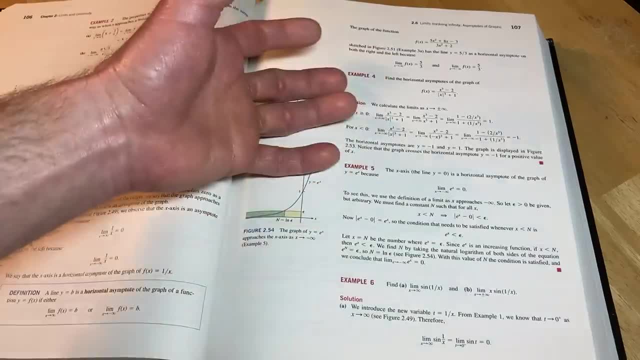 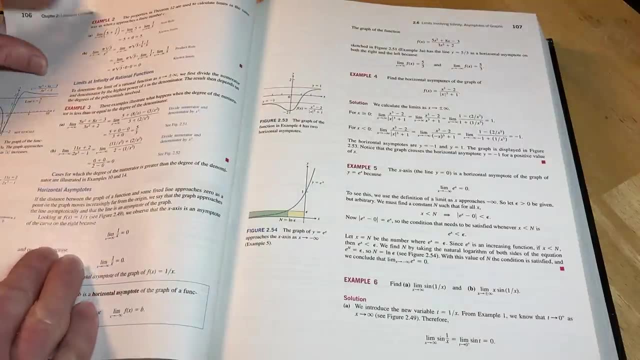 I'm just going to say it's different and it's good and it's worth having newer additions and older. So I'll leave a link in the description so you can check it out. I'm not going to say it's If you want to, But look at all these examples. So this is 2.6, Limits Involving Infinity. 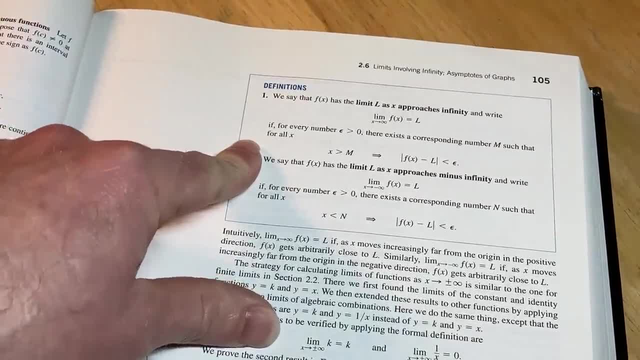 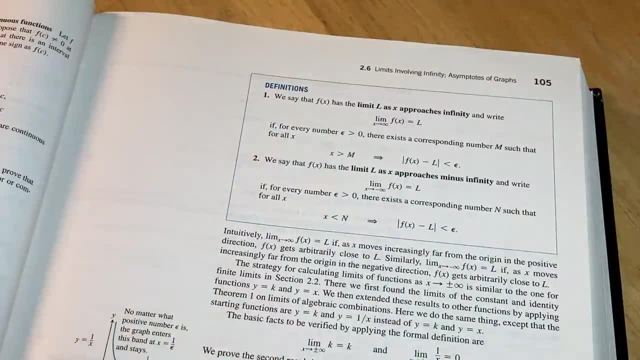 And so they start by giving you the actual rigorous definition, right? So they're not just watering it down or anything. with the updates, It's still a calculus book, right? This is a real calculus book. You're getting real mathematics here. Then they have some examples. 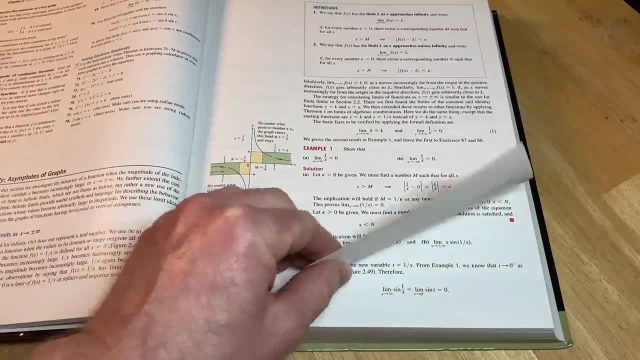 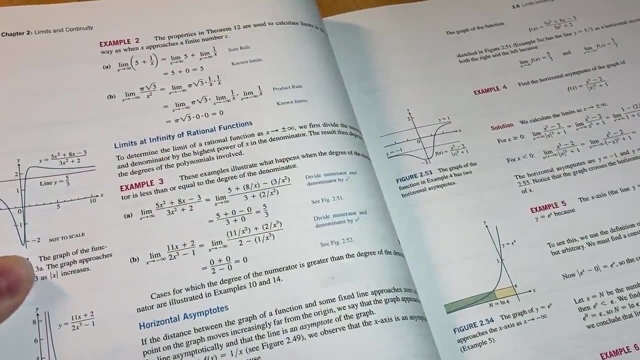 and you can see these examples are proofs with the definition. So it's not like the newer editions, you know, watered it down. It's not like the newer editions, you know, watered it down. The rigor is maintained in many places. And then you see more examples here. Really nice example. 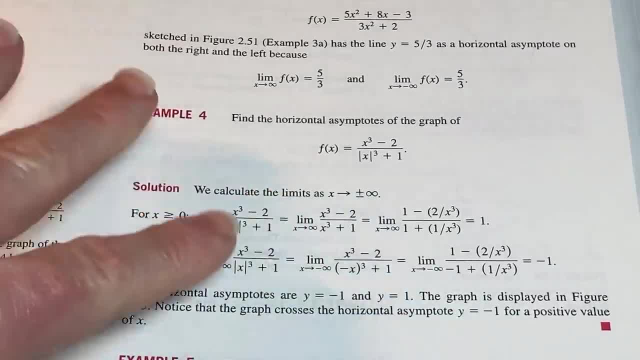 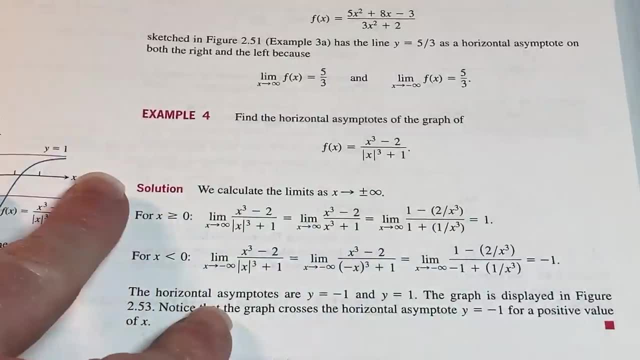 here. Look at this one. It's got an absolute value. That's pretty cool. So there's a lot of things- and it's little stuff like this throughout the book- that I think make this book special. You get examples that you don't see in other books, And that's why I want to recommend this one. 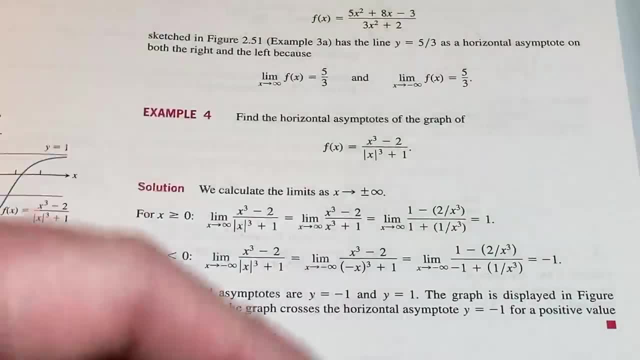 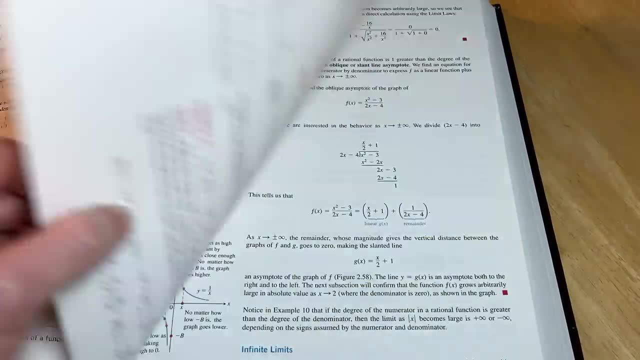 because you're probably using one of those other ones by Stewart or by Larson. So this one's going to give you a different perspective on the subject And different exercises too. This one has answers to all of the odd-numbered problems in the back. 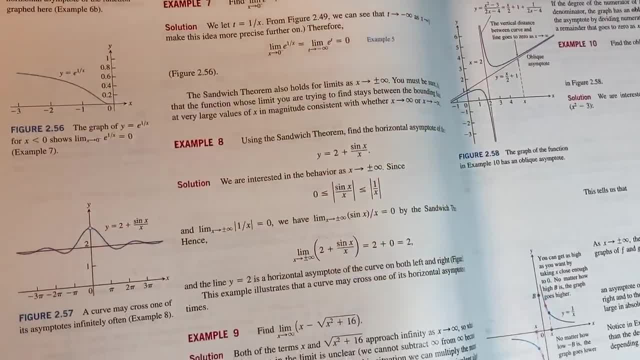 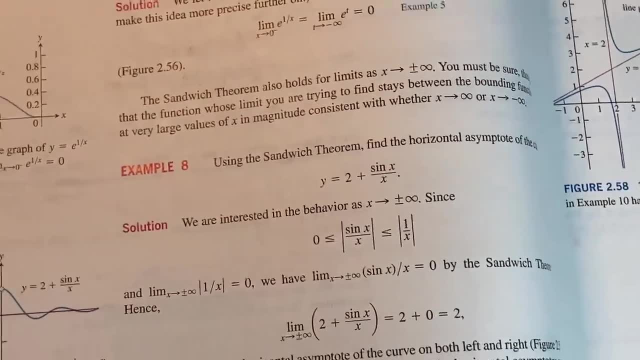 of the book. Look at all of these examples. Oh, I love how they call it. Look at that Using the sandwich theorem. So it's also called the squeeze theorem or the pinching theorem. I don't like that name. I don't like pinching. That doesn't sound comfortable. Oblique asymptotes, which are also: 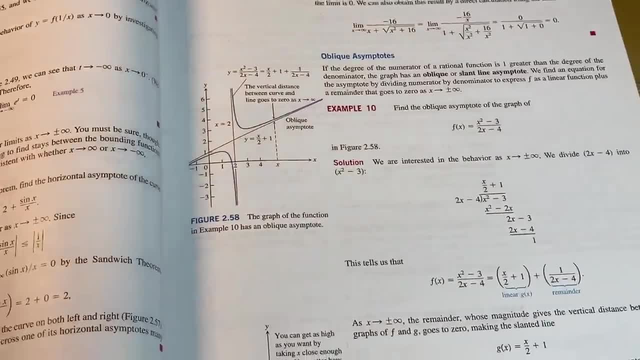 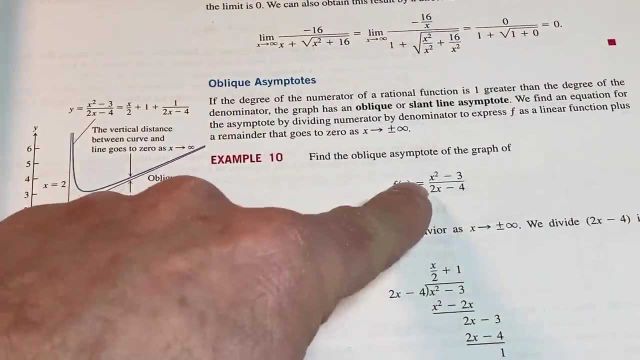 called slant asymptotes. You're asked to find one there. Pretty cool. A rational function will have an oblique asymptote when the degree is exactly one higher. See how the degree in the numerator is two and the degree is one. The degree is the biggest exponent, So 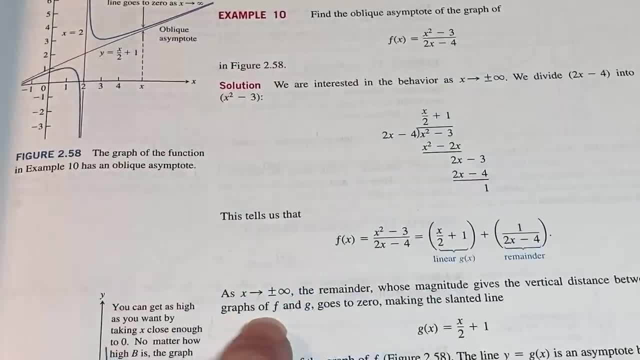 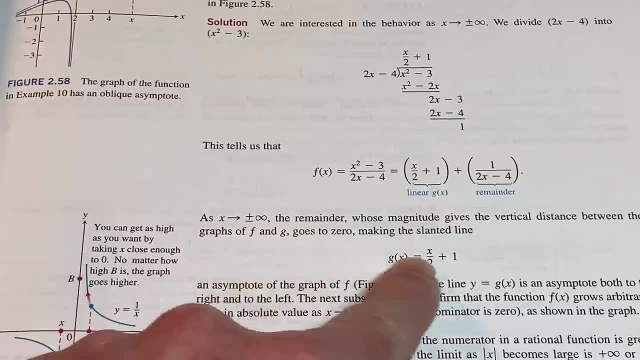 here's two and here's one. So whenever that happens, you can use long division and find the oblique asymptote, And you can see here it even explains it- As x approaches plus or minus infinity, the remainder, whose magnitude gives the vertical distance between the graphs of f and g. 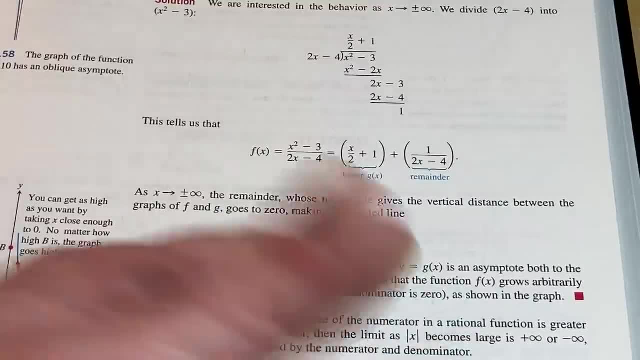 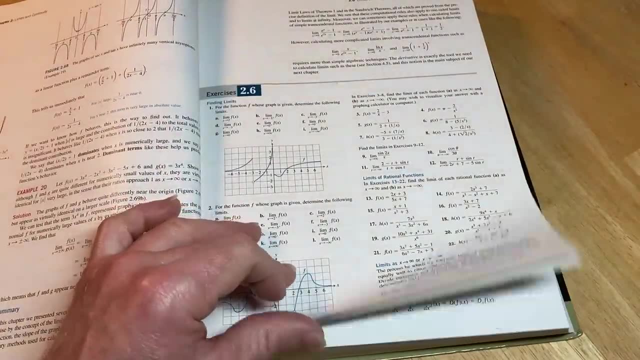 goes to zero, making the slanted line Boom, The oblique asymptote or the slant asymptote. So it explains really well. It's a really good calculus book. Is it perfect? No, But I think you can find copies really inexpensively, especially used copies. 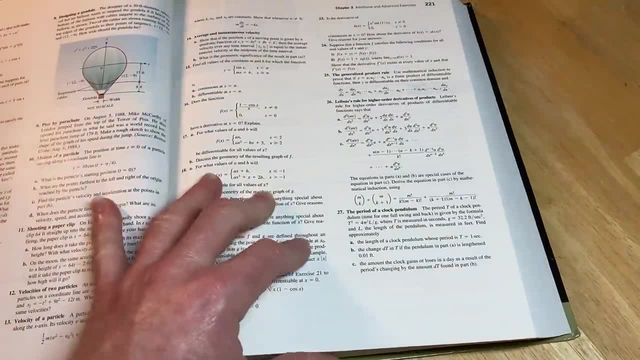 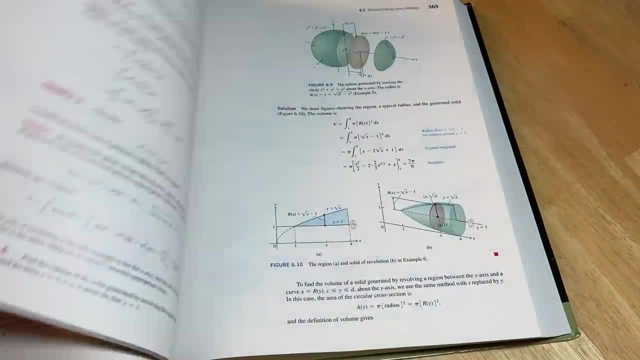 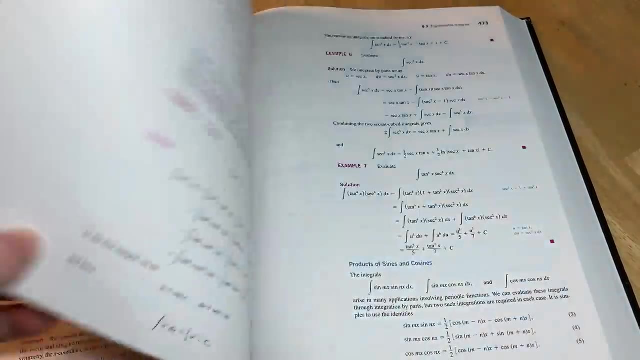 which I think make it worth it. And does it matter which edition you get? I don't think so. My advice would be: get a copy that is inexpensive. You'll probably find less typos in newer editions and less mistakes. I think I might have found a mistake in one of the older editions I have. 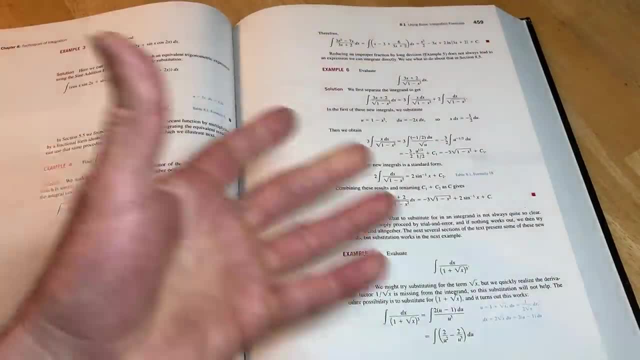 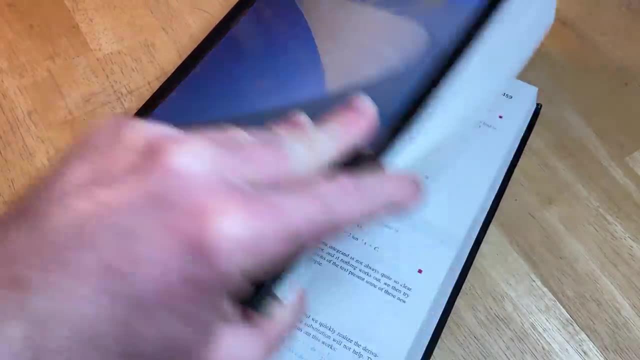 It's like a really old one where the pages are yellowing. I haven't seen any errors in this particular edition. This one's the 13th And again I'll leave a link or two in the description to various used copies, And I would just recommend getting a used copy right- A used copy or a new. 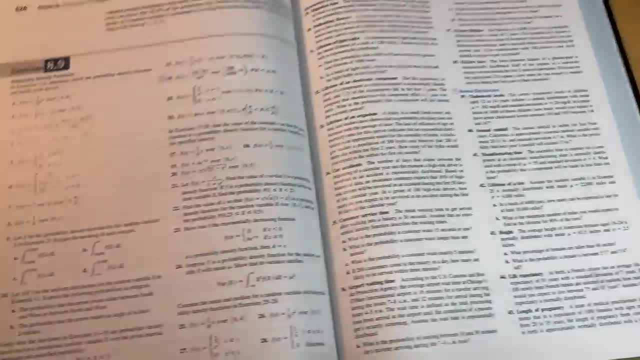 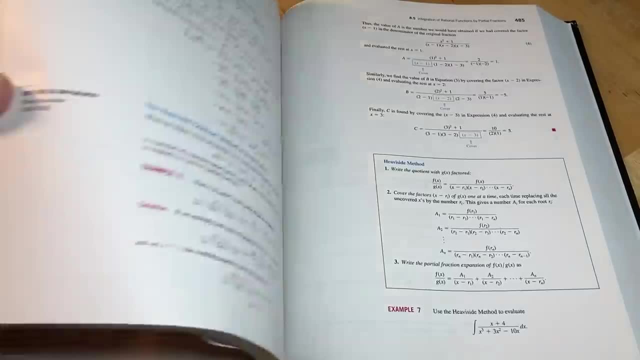 one, if you want, of this great book. And how do you use this book? Well, so you have a calculus book and you want to learn calculus, So my advice would be to try to do a little bit every day. at least one problem a day If you're already learning calculus. 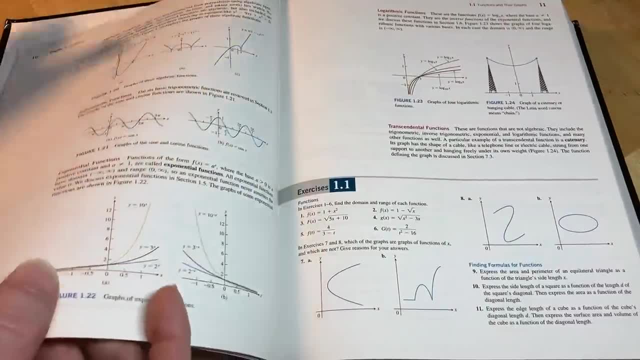 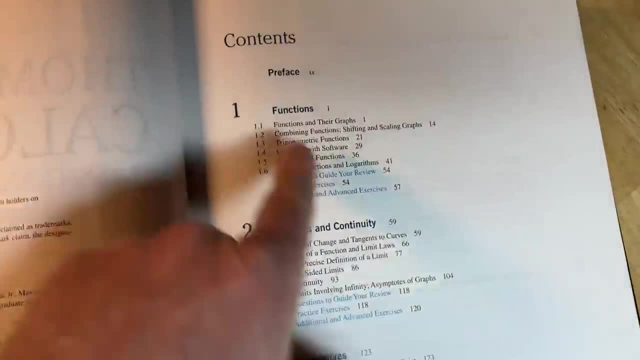 you can easily, easily, easily find what you're learning in the book by looking in the contents. Let me just show you the contents really quick. I forgot to show you So functions. it's the basic stuff, right? It's all the stuff that you would typically. 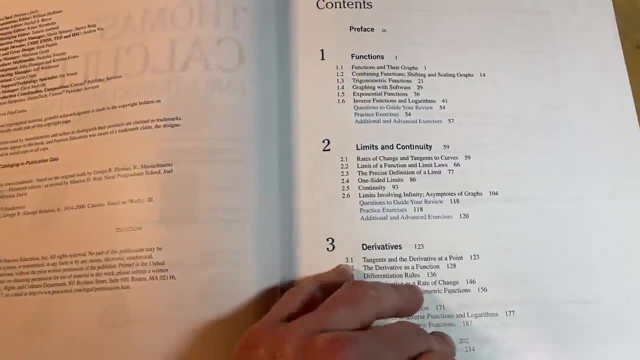 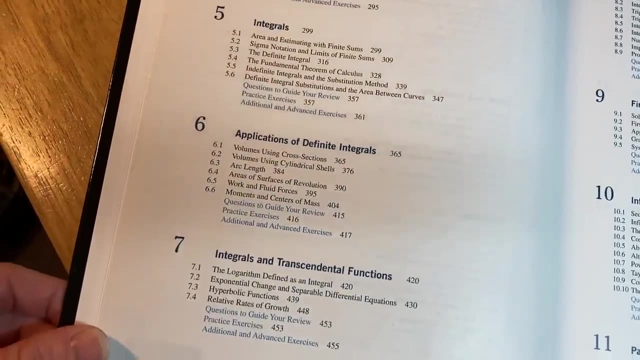 see in a calculus class. So it's all the same topics. The order is very similar. I mean: look, applicate, it's just, you know, boilerplate, as they say. right, Everything you would see in a calc course. 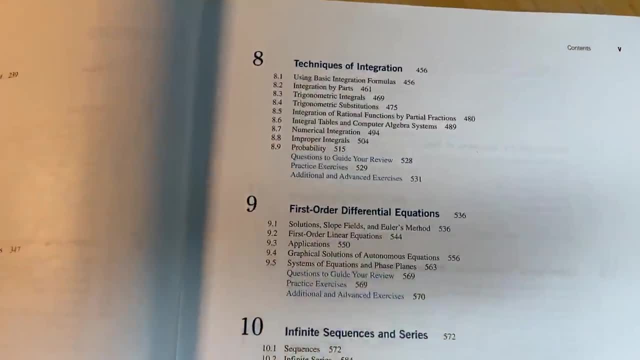 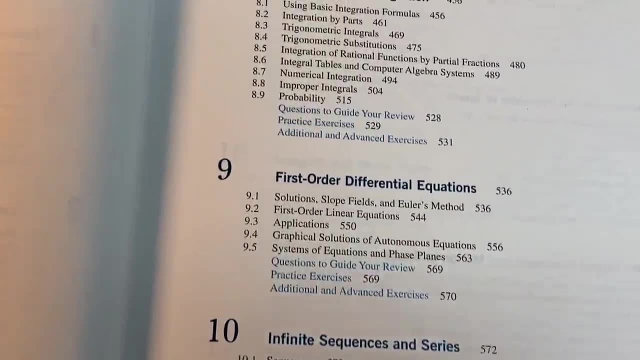 It's even got the differential equations in there, The standard techniques, all the standard techniques for integration. So everything you would see, although it does have a section on probability, which a lot of books do have, but it's typically not something that's covered. 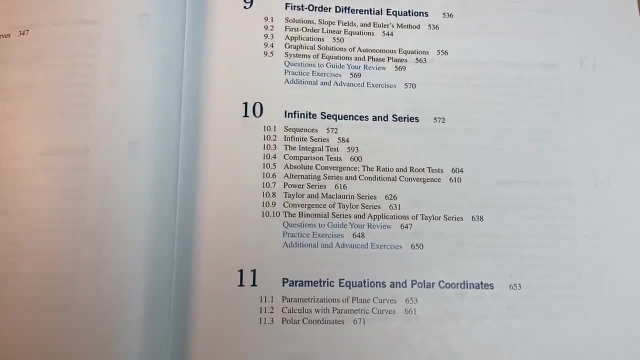 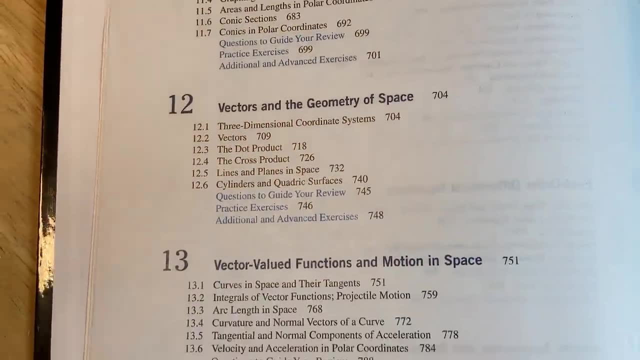 That's not something you'll learn if you take a college level course. Typically, your teacher will not spend time on that, Not because they don't want to or they don't like it- which could be true- but it's because of time constraints. Typically when you're a teacher. 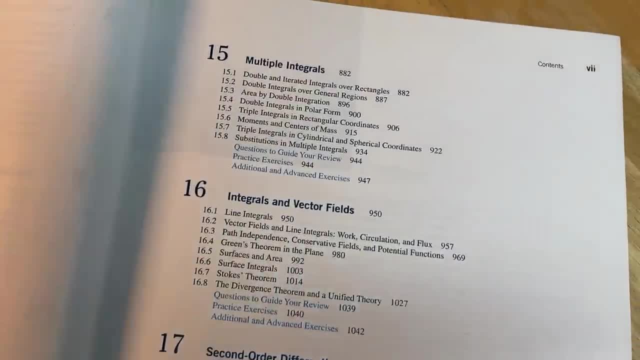 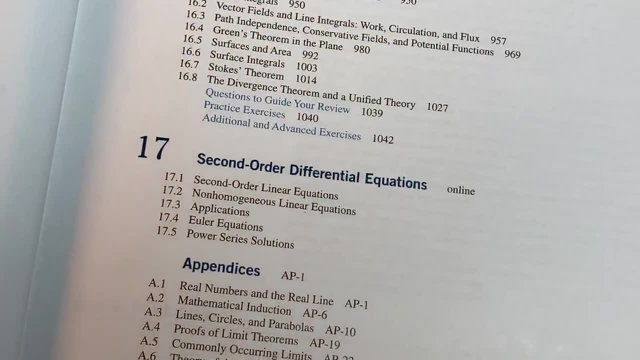 teach certain topics, So your goal is to cover those topics. Yeah, integrals and vector fields- This is Calc 3 stuff. And then second order, DE, is typically not covered. I personally have never taught this, and I've taught Calc 1,, 2, and 3 multiple times at colleges. 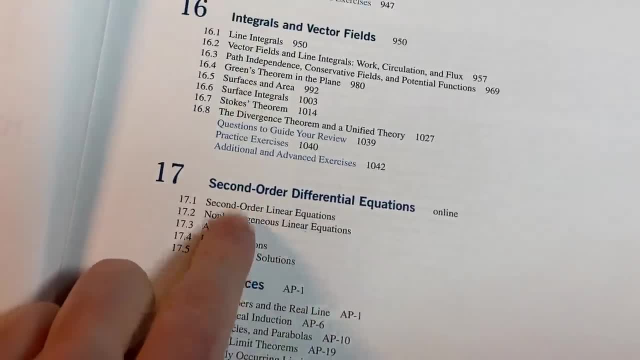 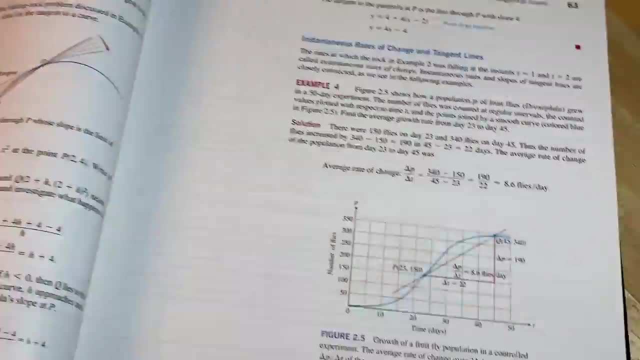 Answers to odd-numbered exercises. Yeah, this is taught typically in differential equations. Yeah, it's a great book. It's a great book. It really, really is. I'm just going to have to give it a whiff here, because I love this book. This is really good. I want to thank the 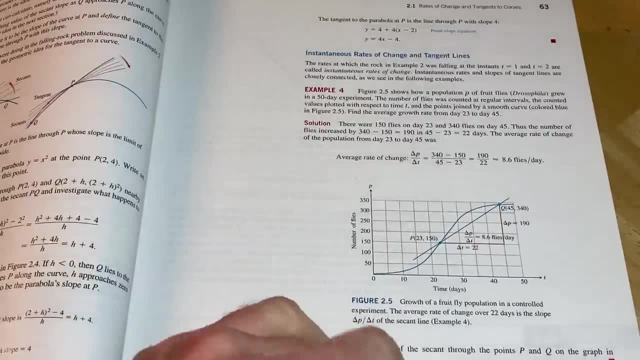 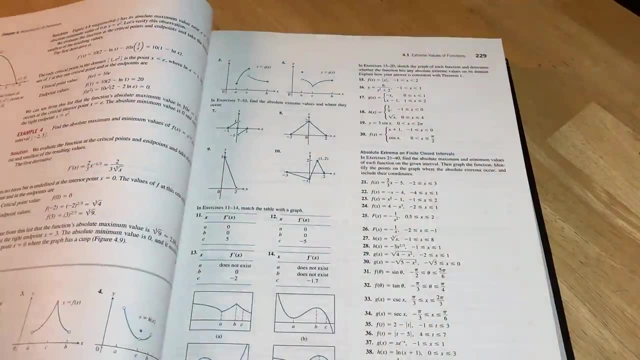 subscribers too, who mentioned this book. They kept mentioning it because I made a video on the Stewart book and then people were like, oh, what about Thomas Calculus? I'm like Thomas Calculus, what's that? And so it's been a while and I bought it And, yeah, I like it. I think it's. 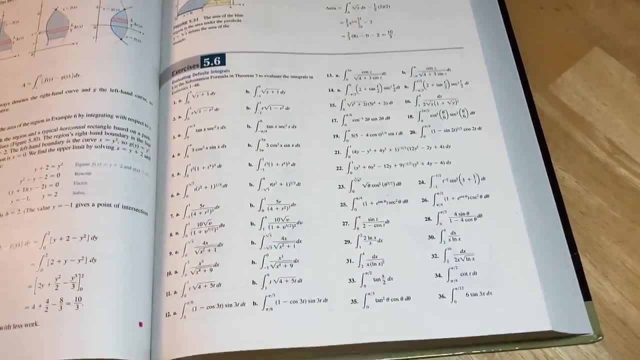 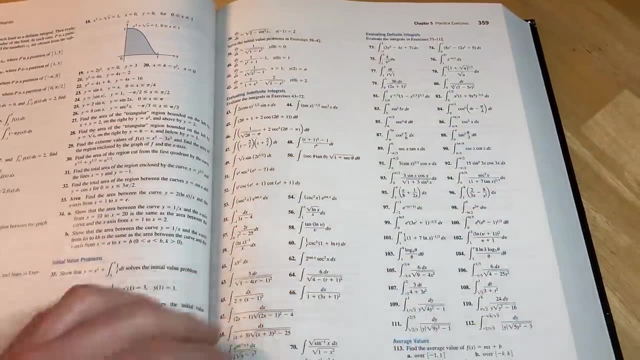 a great book. It's thick. Look at all these exercises too. Look at this. It's ridiculous, Ridiculous. how many problems you get here, right? I mean? so many examples, so many exercises, So wow, right. 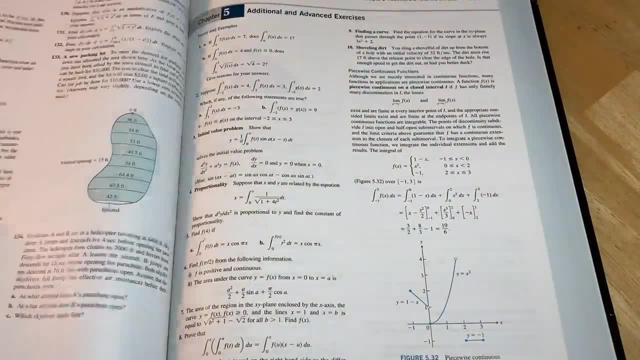 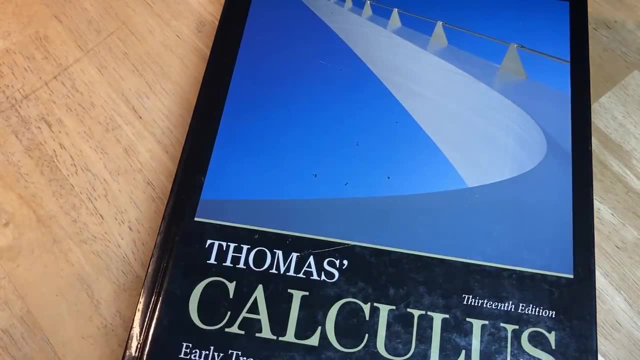 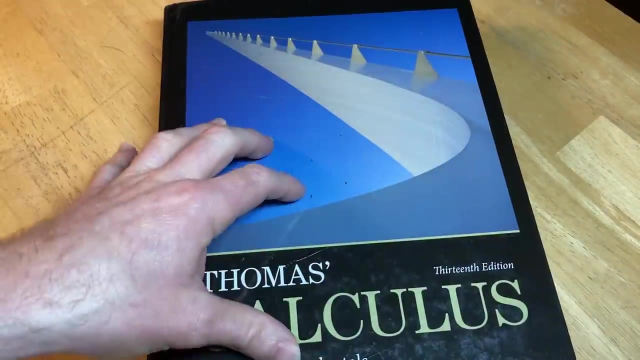 Tons of problems, Super awesome, Really really good stuff. Yeah, it's awesome. Anyways, great book. I recommend it Also if you want to learn math through a course, which is another way to learn calculus. I do have courses on my website, mathsourcercom. They're actually on. 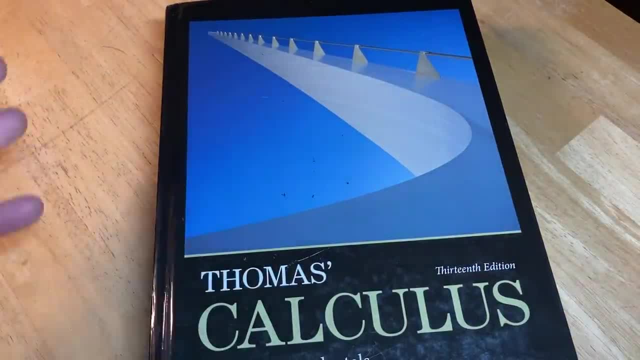 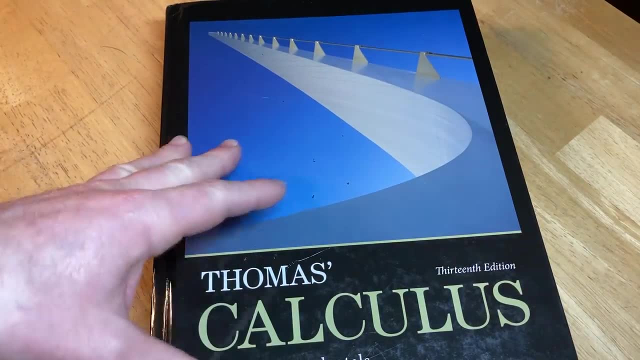 the Udemy platform. so it's a reputable place and they have a good platform. But if you decide to get my courses, please go through my website or the links in the description- mathsourcercom, as it helps me greatly And I've lowered the prices to make them as low as Udemy. let me make. 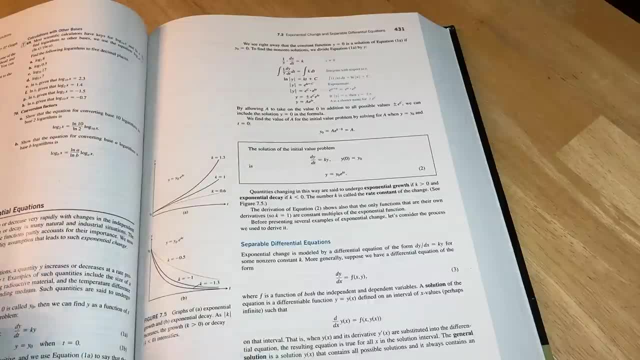 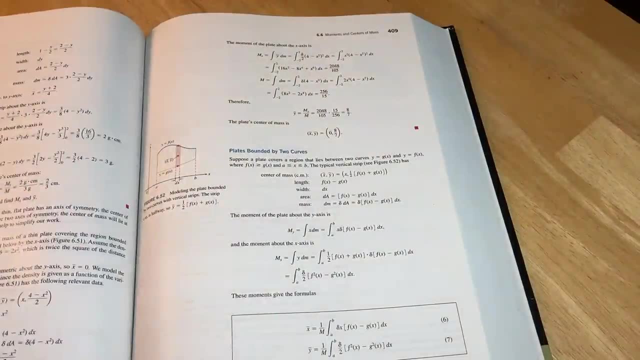 them, so I set them to the bare minimum. So if you use my links, you'll help me and you should get a low price. And if you found any value in this content and you want to subscribe, subscribe if you want to. If not, that's okay too. Oh, look moments. Ooh, got distracted. Calc 2 stuff, This.